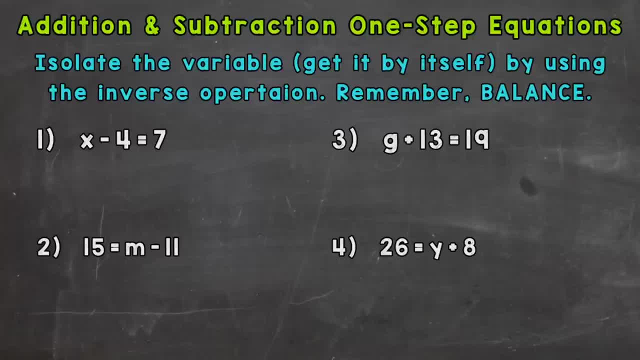 So at the top of the screen is a very important note. We need to isolate the variable, which means get it by itself by using the inverse operation. Inverse operation means opposite operation And we have to remember to keep everything balanced. So let's see exactly. 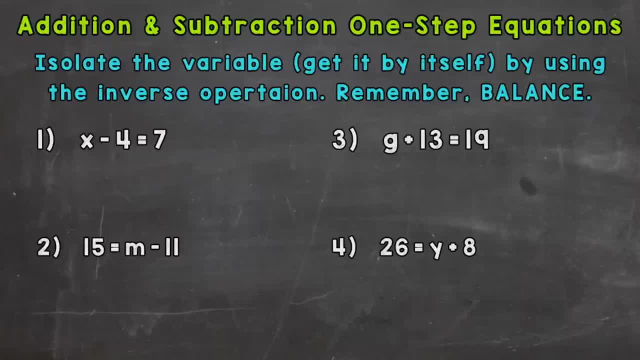 What that means. as we go through our four examples here, starting with number one, where we have X minus four equals seven. X is our variable that we need to isolate, and we are subtracting four from X. So the inverse or opposite operation would be to add four. 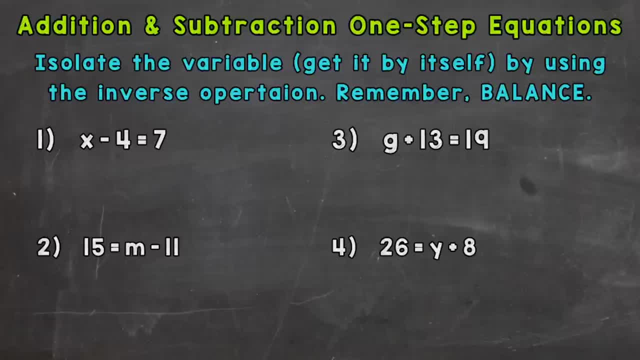 So let's add four to that side. That way the fours cancel out. So we have a subtraction of four and an addition of four. So those fours cancel out. But remember, keep everything balanced. So whatever we do to one side, we have to do to the other. 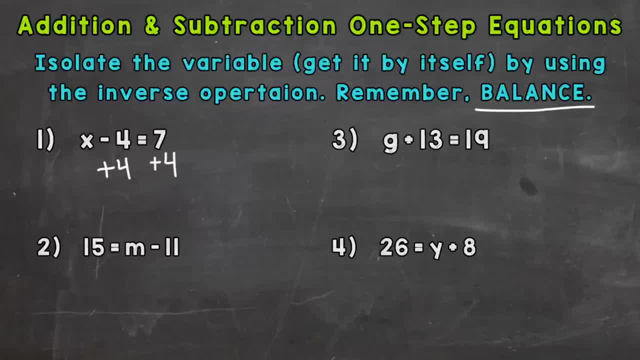 So let's add four to the other side as well. So the fours on the left cancel each other out, leaving X by itself. We isolated that variable. Now, seven plus four on the right will give us eleven. So X equals eleven. 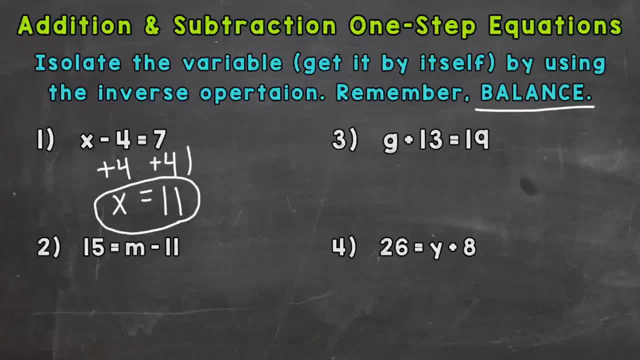 And we can double check that we have the correct answer by plugging the eleven back into the equation. So eleven minus four equals seven, which is true. So we have the correct answer there. X equals eleven. Now number two: we have an equation there that looks a little different than number one, because we have the fifteen on the left and then the M minus eleven, the variable on the right. 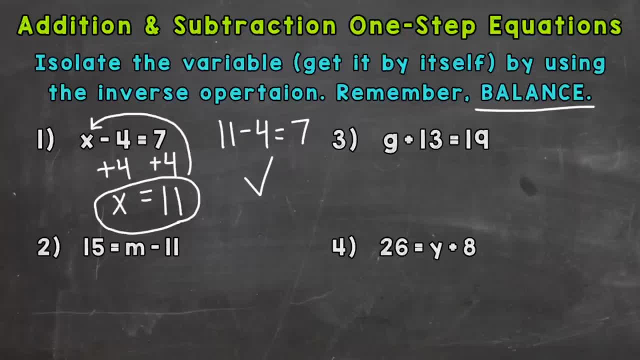 Although it looks a little different, it's the same exact process. So we need to isolate the variable, the M. We are subtracting eleven, So what's the opposite of subtracting eleven? Well, adding eleven. So let's add eleven to that side. 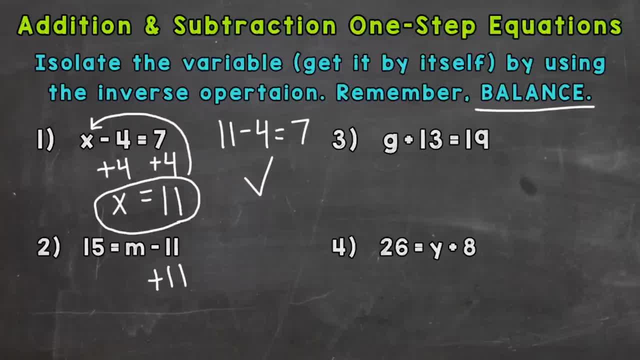 That way, those elevens cancel out and the M is left by itself. Now, whatever we do to one side, we have to do to the other. So M is by itself, And fifteen plus eleven, well, that equals twenty-six. 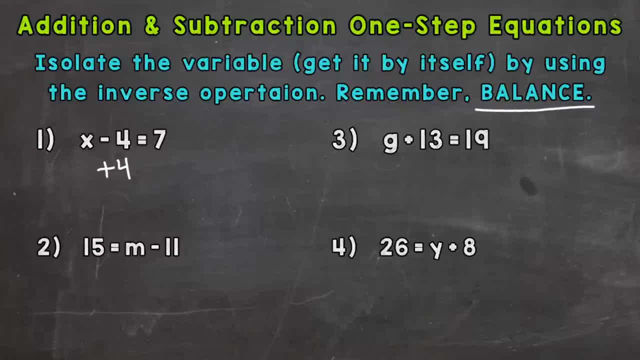 keep everything balanced. So whatever we do to one side, we have to do to the other. So let's add four to the other side as well. So the fours on the left cancel each other out, leaving X by itself. We isolated that variable. Now, seven plus four on the right will give us 11.. So X equals 11. And we can double. 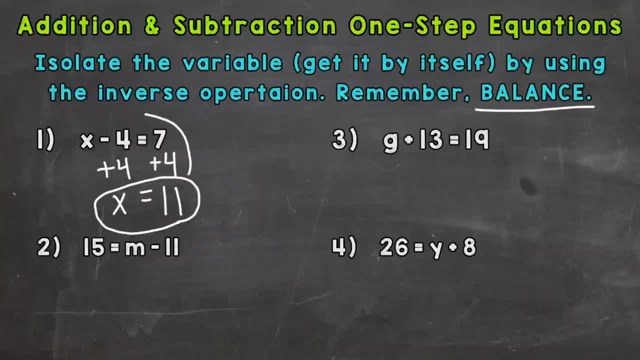 check that we have the correct answer by plugging the 11 back into the equation: 11 minus four equals seven, which is true, So we have the correct answer there: X equals 11.. Now number two: we have an equation there that looks a little different than number one. 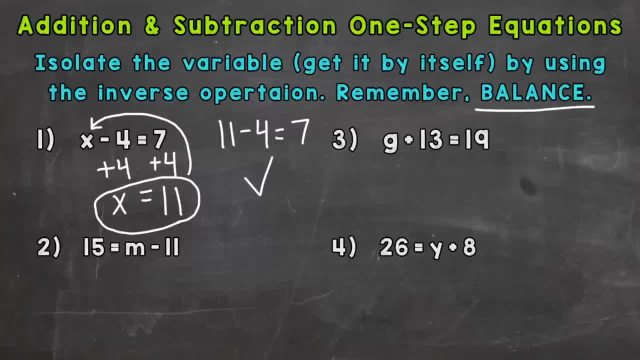 because we have the 15 on the left and then the M minus 11, the variable on the right. Although it looks a little different, it's the same exact process. So we need to isolate the variable, the M. We are subtracting 11.. 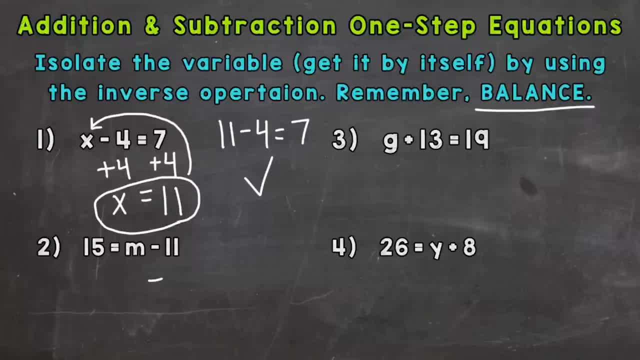 What's the opposite of subtracting 11?? Well, adding 11.. So let's add 11 to that side. That way, those 11s cancel out and the M is left by itself. Now, whatever we do, to one side. 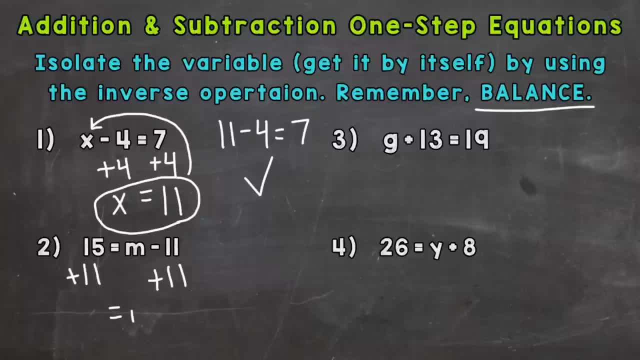 we have to do to the other. So M is by itself, And 15 plus 11, well, that equals 26.. So M equals 26. And we'll plug back in to see if that's true. So 15 equals. 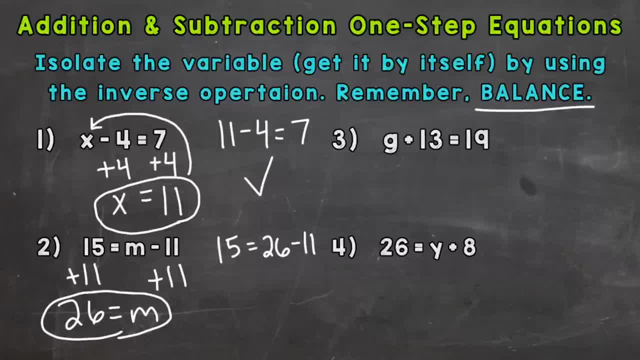 26 minus 11, which is true, And you can think of these equations like balancing a scale. Both sides need to be exactly equal. So on the left we have 15, and 26 minus 11 equals 15 as well. 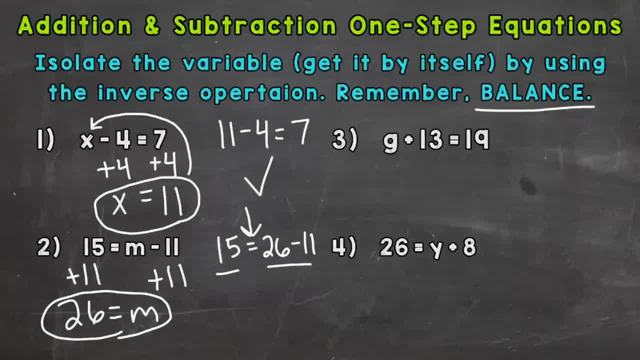 So both sides are exactly equal. On to number three, where we have G plus 13 equals 19.. So we need to isolate the G, the variable, We are adding 13.. So the opposite of adding 13 would be subtracting 13.. That way those 13s cancel out. But remember: 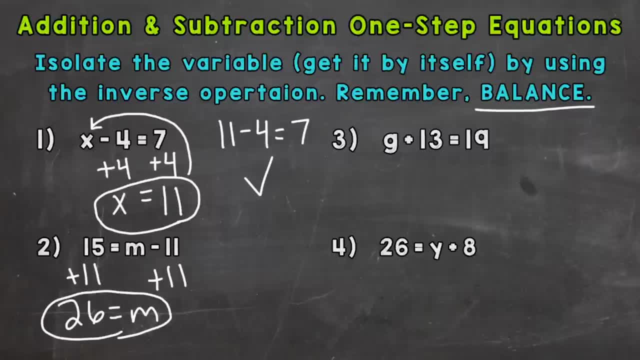 So M equals twenty-six, And we'll plug back in to see if that's true. So fifteen plus eleven equals twenty-six. So fifteen plus eleven equals twenty-six. So fifteen equals twenty-six minus eleven, which is true, And you can think of these equations like balancing a scale. 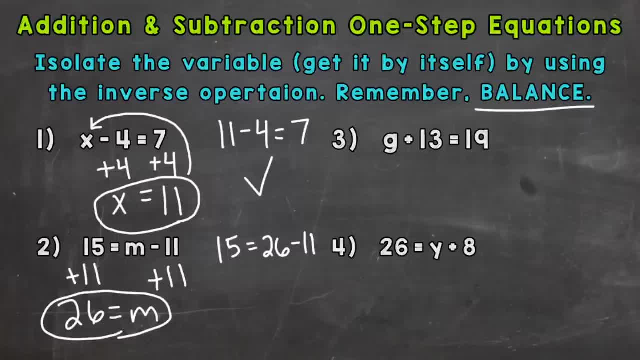 Both sides need to be exactly equal. So on the left we have fifteen And twenty-six minus eleven equals fifteen as well, So both sides are exactly equal. On to number three, where we have G plus thirteen equals nineteen. So we need to isolate the G. 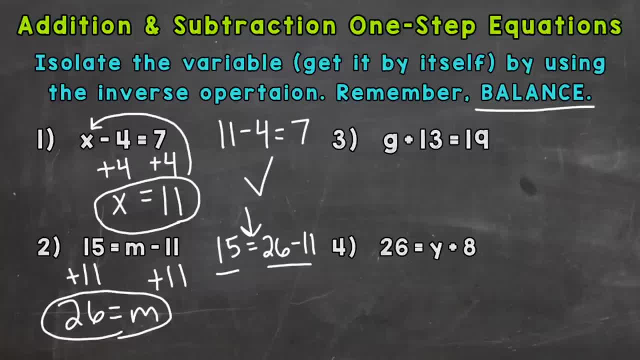 The variable, We are adding thirteen. So the opposite of adding thirteen would be subtracting thirteen. That way those thirteens cancel out. But remember, whatever we do to one side, we have to do to the other. So subtract thirteen from the right. 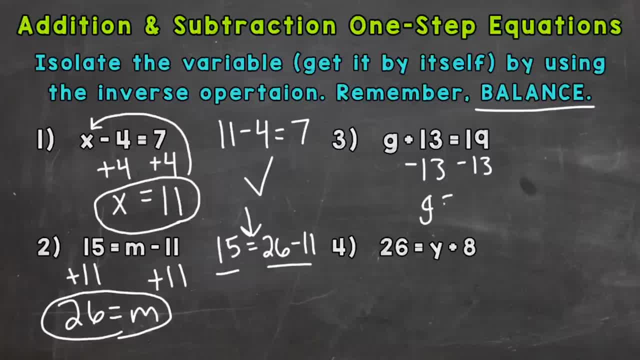 That nineteen. over there, G is now isolated And we have nineteen minus thirteen, which gives us six. So G equals six And we'll plug back in Six plus thirteen. Thirteen equals nineteen. So that's true And we have the correct answer. 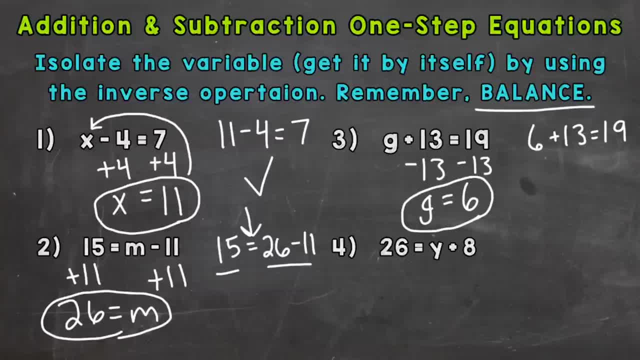 On to number four, where we have twenty-six equals Y plus eight, So we're adding eight to the variable Y. We need to use the inverse or opposite operation. So subtract eight. That way we isolate Y. Whatever we do to one side, we do to the other. 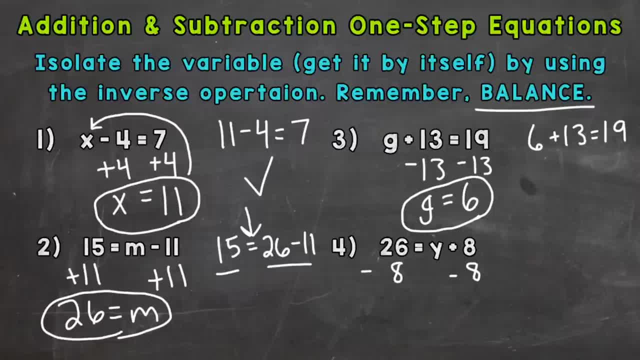 So let's subtract eight from the left as well. Y is now isolated, And twenty-six minus eight equals eighteen, So Y equals eighteen. Let's plug back in and see if this is true. Eighteen plus eight is twenty-six, So we are good to go with number four.